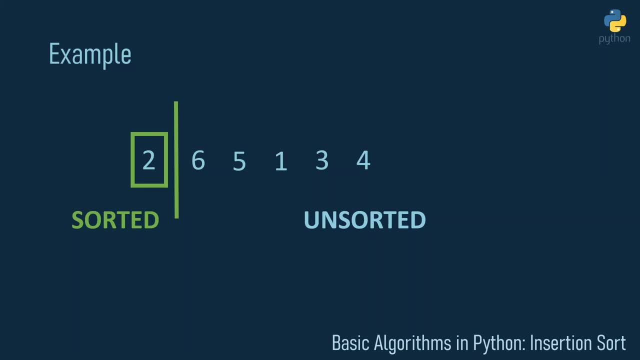 into two parts: an already sorted part and an unsorted part. Before the first iteration, only the first element belongs to the sorted part and we want to extend this sorted part with every iteration. Therefore, insertion sort looks at the first element of the unsorted part. 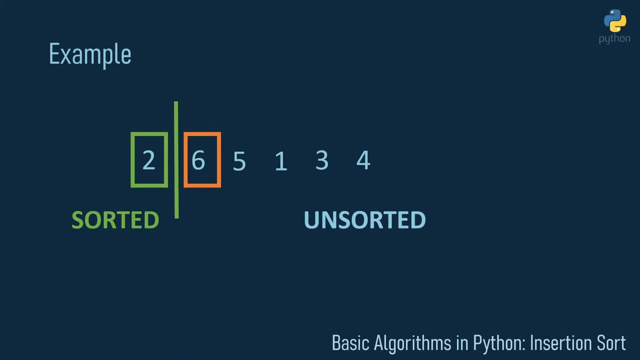 and tries to insert it into the sorted part. This is done by comparing the six in this case to its left neighbor. the two Six is greater than two, so nothing needs to be done in this case. In the next iteration, the five needs to be inserted into the already sorted part. 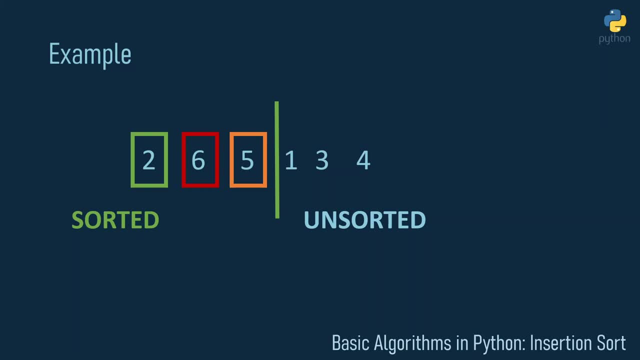 therefore five is again compared to its left neighbor, The six. five is less than six, so in this case insertion sort swaps these two numbers And the next comparison will happen between the five and the two, and in this case five is larger than two, so there's no swapping. In the next iteration, the one of the unsorted part is compared. 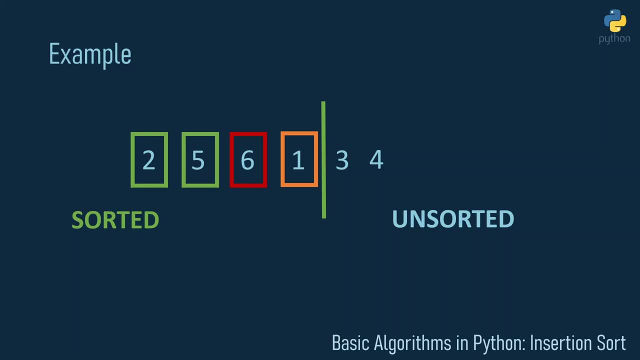 to the six of the sorted part, and those numbers are swapped because one is less than six. Then the comparison goes on between one and five. One is less than five, so these numbers are swapped again. and the next comparison is between one and two. One is less than two, so there is another swap. 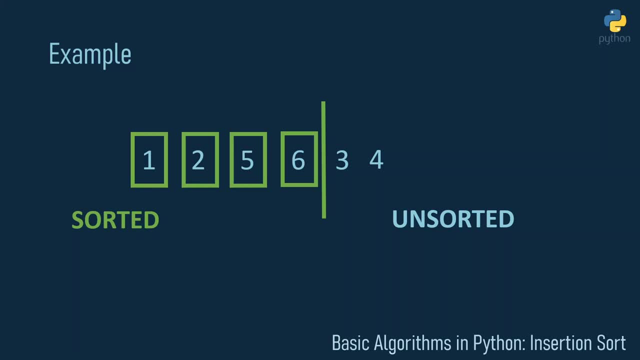 This leaves us with an already sorted list of one, two, five and six, and we can continue with the next iteration And the three. the three is compared to its left neighbor, the six. Three is less than six, so there's a swap. and again, three is less than five, so there's another swap. 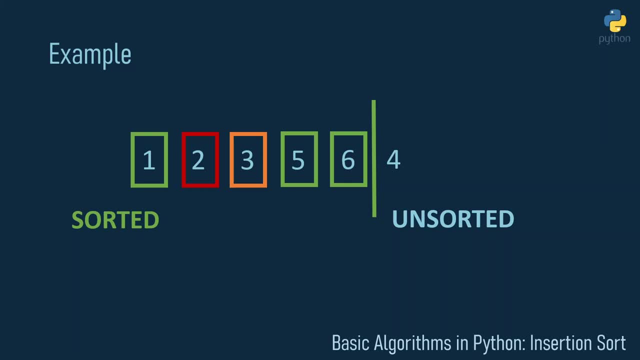 This inner iteration then ends here, because three is greater than two, so nothing is to do, and we are already at the last iteration of this algorithm and this last iteration just tries to fit in the four into the sorted part part. Therefore, 4 is compared to 6, 4 is less than 6, so there's a swap. 4 is 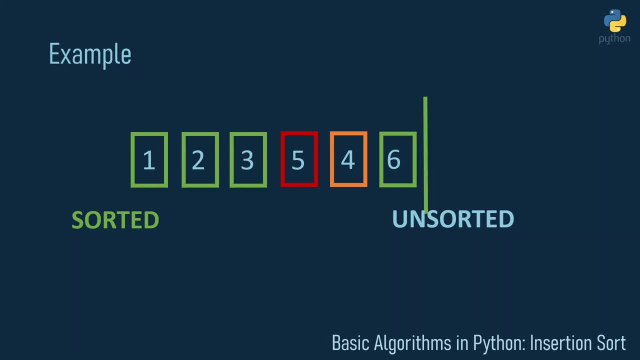 compared to 5, 4 is less than 5, so there's a swap, And this iteration ends here, because 4 is bigger than 3 and we end up with a perfectly ordered list. I hope this example helped you to understand what the algorithm does, and I 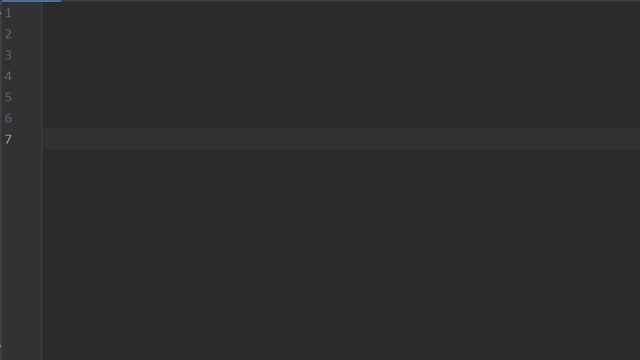 think we're now ready to start with the implementation in Python. First of all, let me define our list in Python so that we have something to test our implementation on. I think it was something like this: You can always define a list in Python with square brackets. 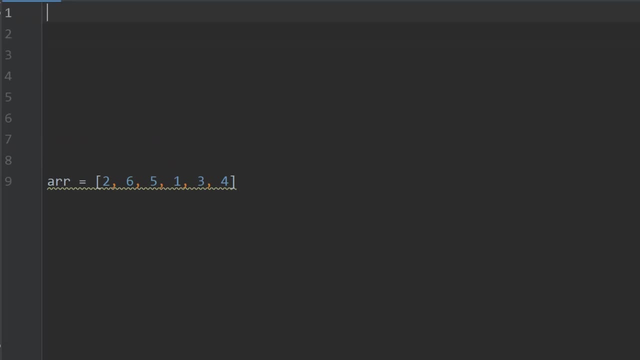 And now for the algorithm. I want to define a new function with the def keyword. The function is called insertion, sort and the parameter array is passed. Now for the algorithm. we need an outer loop that goes from the second element to the last element. So we want to iterate through. 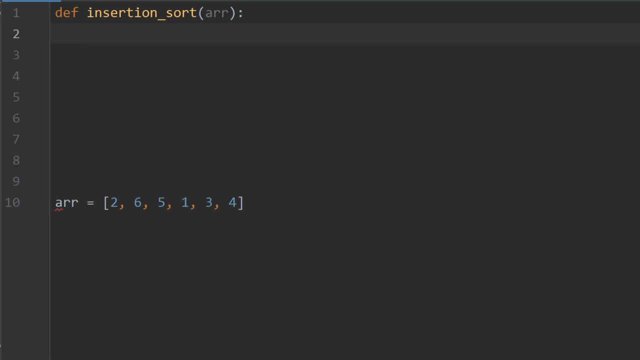 all unsorted items. Therefore, I use a for loop. This for loop gives us the index 1 to length of array. Length of array in this case is 6. And this range function excludes the last index, so we really get the indexes 1 to 5.. The indexes 1 to 5 in this example array point at the 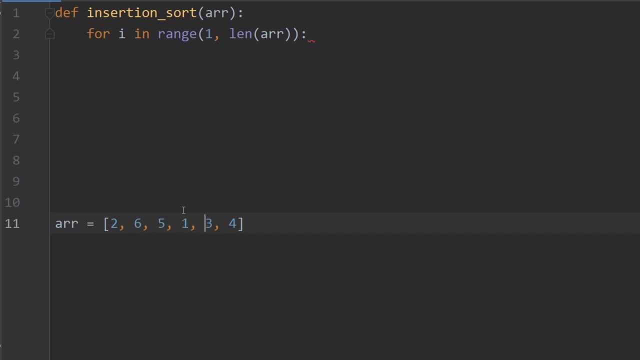 entries in the list 6,, 5,, 1, 3 and 4.. And now we need an inner loop that starts at the index of the outer loop and iterates the list to the left and checks if we need to do swaps and stops if we don't need to swap anymore, If the right place. 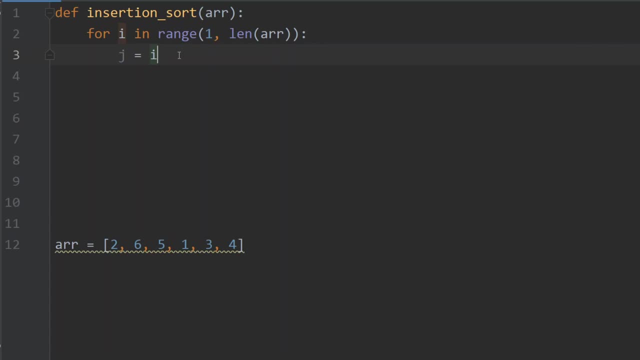 for a current number is found. So this inner loop needs some condition. The first condition is our swapping condition, And our swapping condition looks like something like this: We want to check if the left neighbor is bigger than the current element And in this case we want to do a swap And swaps in.